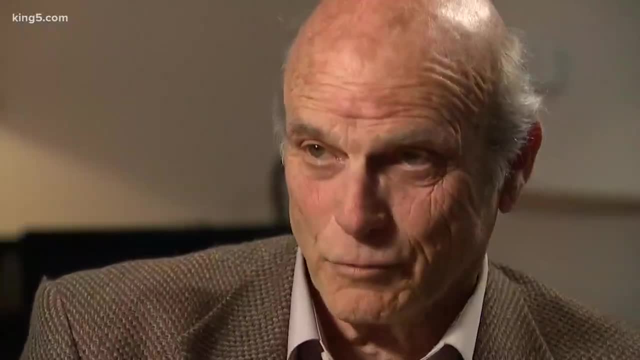 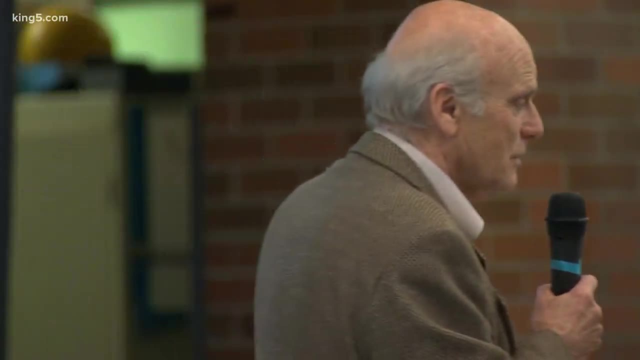 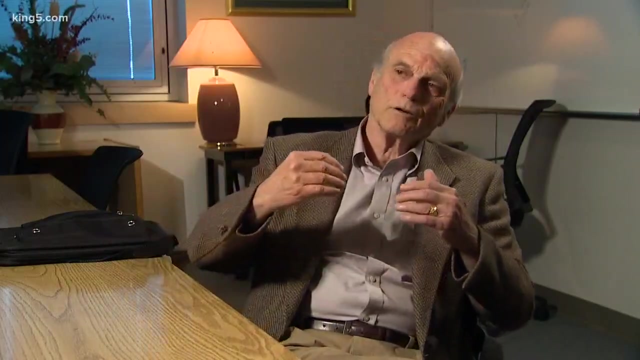 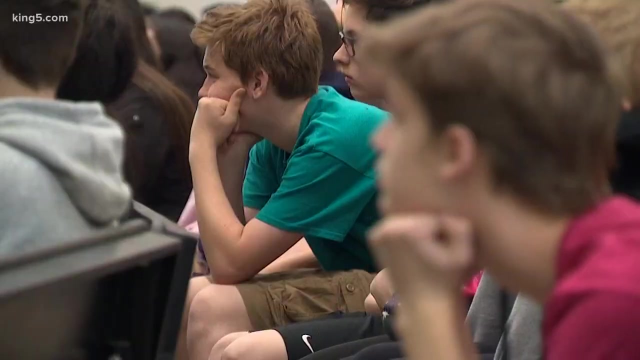 Holocaust is the first of many levels of the Holocaust in human history, He told. I'm not sure I'm a scholar, but I guess you could call them their witnesses. now You know their witnesses to my story. Metzeler testified in favor of the bill so more students would hear stories like his. Something he says is especially needed today. 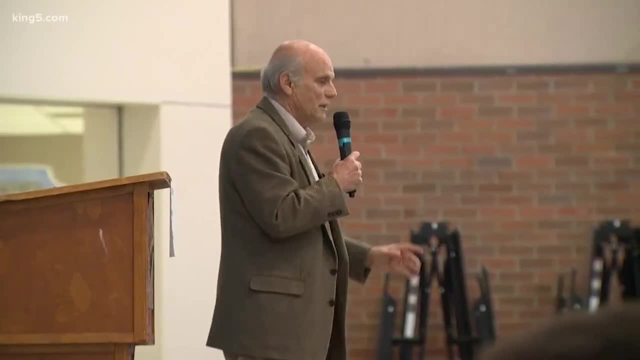 He can truly say that it had to do with Germany and the Jewish people, But you can almost go beyond that in today's setting. What it had to do is what mankind is capable of doing to mankind, And the thing that scared me every time is that this is what we're doing here. 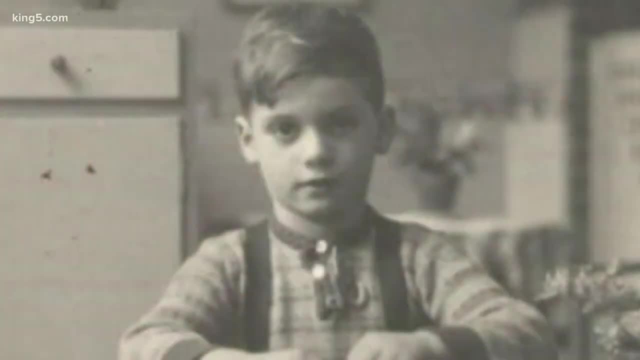 What can you do to save the people in this country? It's the right thing to do. That's the right thing. And it's the right thing to do to save the people in this country. That's the right thing to do. time they're going to come get me, I am so scared He hopes by teaching the dangers of. 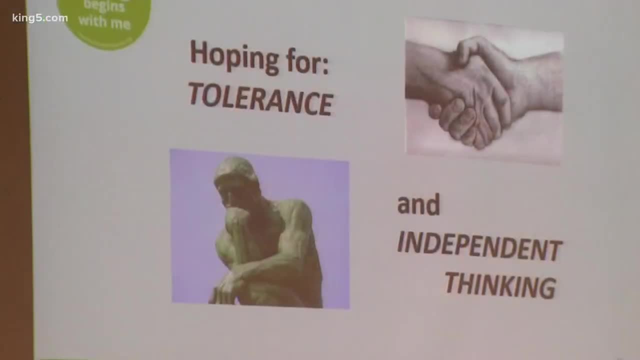 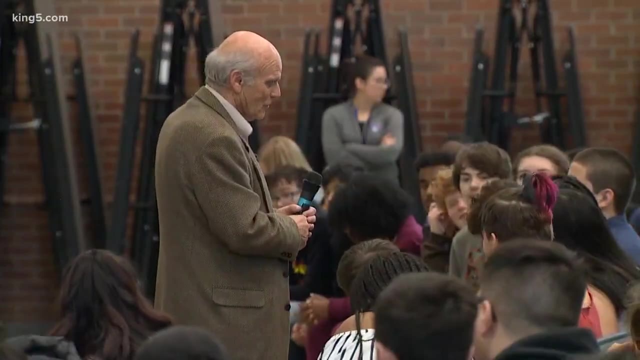 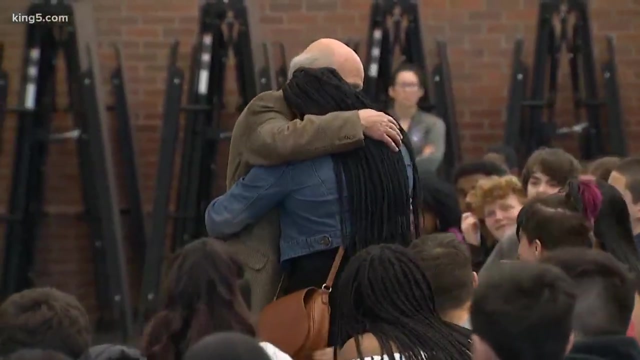 propaganda and intolerance, students will learn hatred is not the answer. It's a message, he says, has an impact every time. You're just not breaking down- and I am, and I didn't even go through any of this- Stand up, Give me a hug. Drew Mickelson King 5 News. 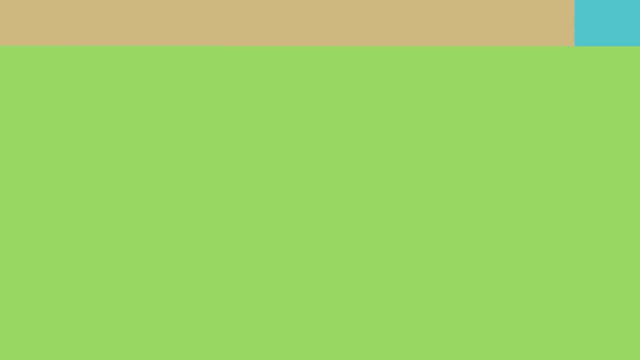 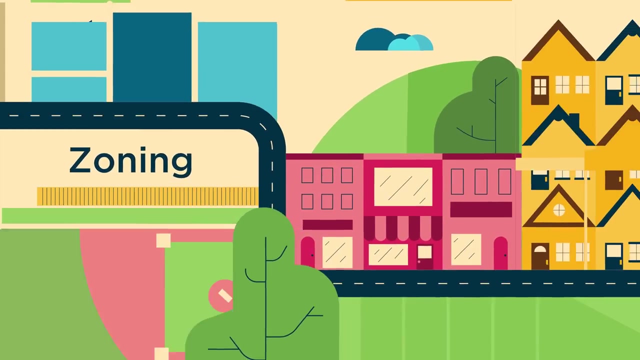 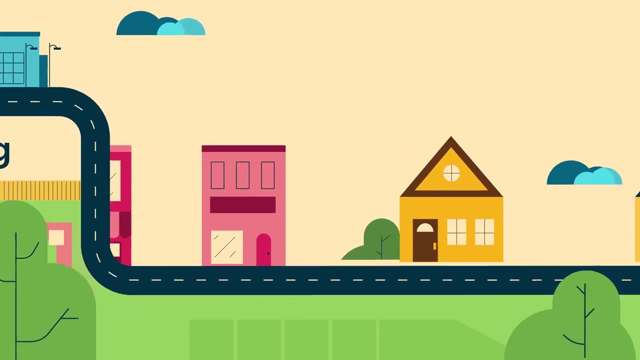 Zoning is a way for communities to separate land by use or form. For example, an area could be dedicated to commercial or industrial use, or there could be a restriction on how many housing units can be built. Zoning shapes the places where we live, but it also shapes our lives. 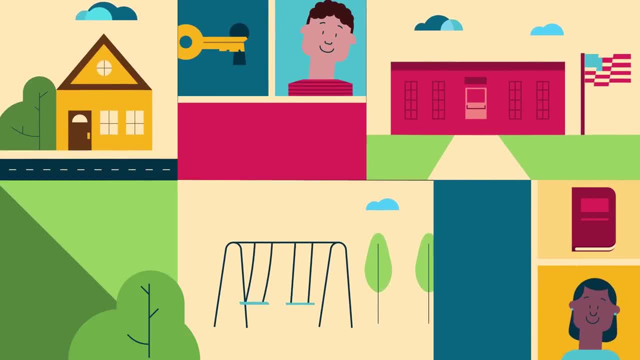 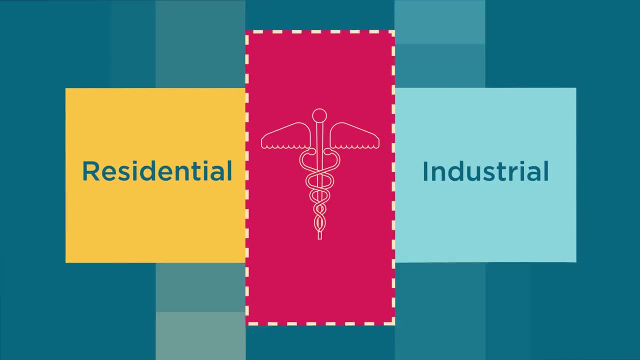 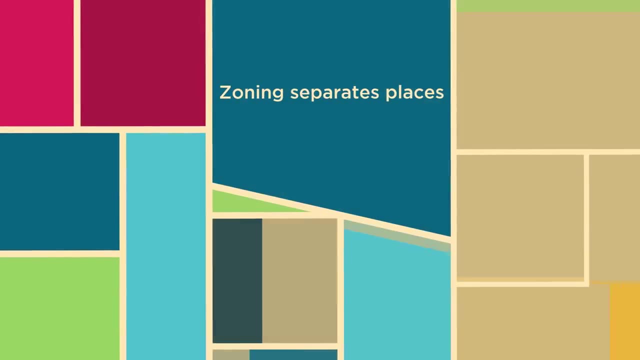 Local zoning regulations determine where we can find housing, schools and parks and who gets to use them. Policymakers initially created zoning codes to protect public health, For example to stop residents from getting sick from living too close to factories. But from the start, zoning has separated more than just land uses. It has also separated people. 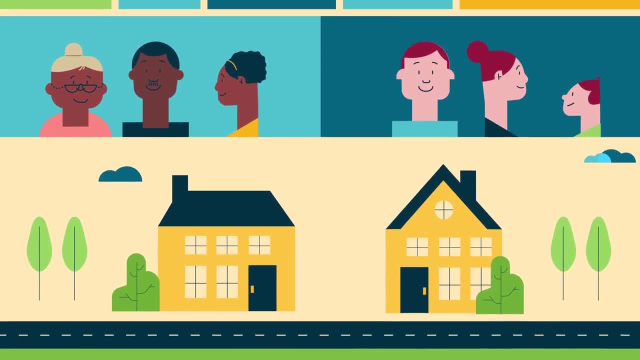 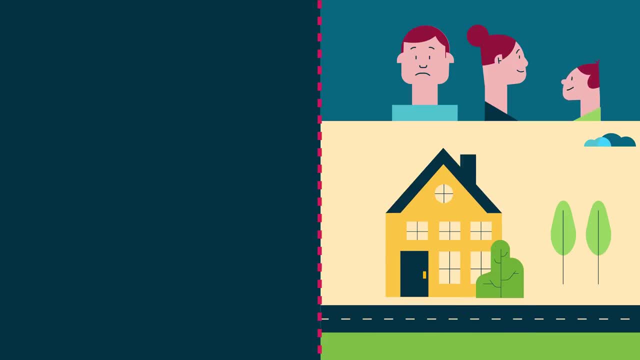 In the early 20th century, many communities explicitly used zoning ordinances to racially segregate neighborhoods, effectively declaring that different skin colors were as incompatible as a family's home and a smokestack. By the late 20th century, civil rights legislation outlawed. 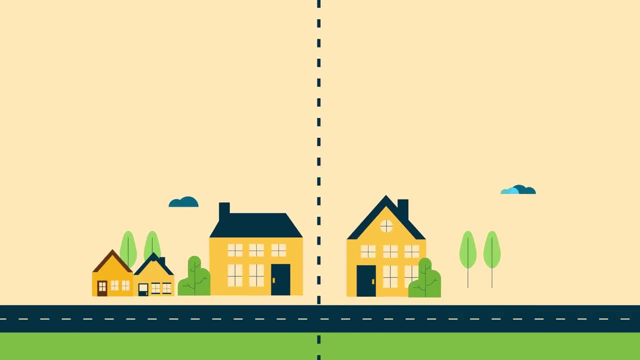 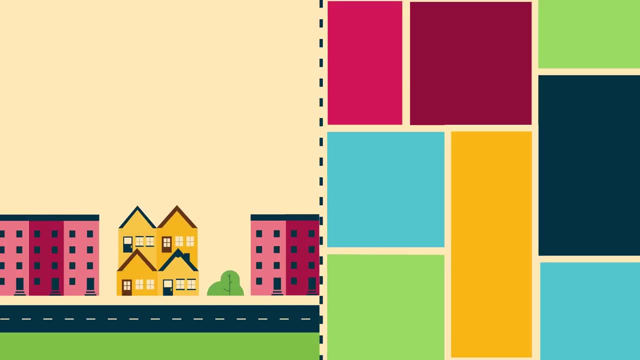 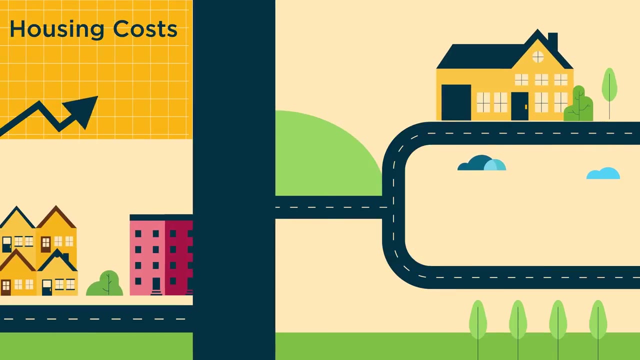 overt housing discrimination. But those explicit racial barriers were quickly replaced by subtler methods. Even today, exclusionary zoning policies that restrict lower cost or higher density housing limit racial and economic diversity and raise housing costs By driving up housing costs. restrictive zoning can exclude: